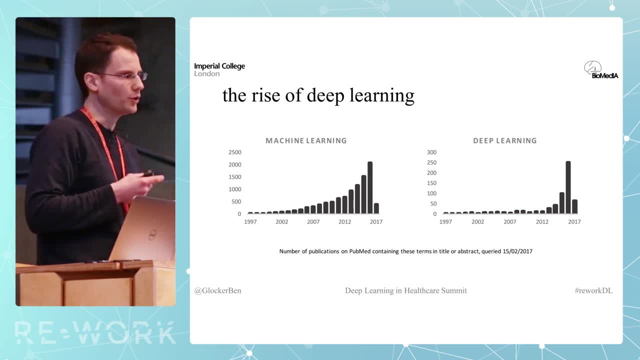 driven approaches. However, if you do something similar with deep learning, it's less of this trend, It's more of a disruption. So you basically see there wasn't much at all And then, very suddenly, there was this huge jump in the number of publications. So, a few years. 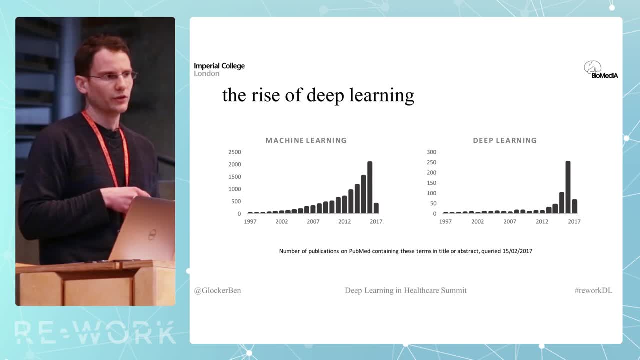 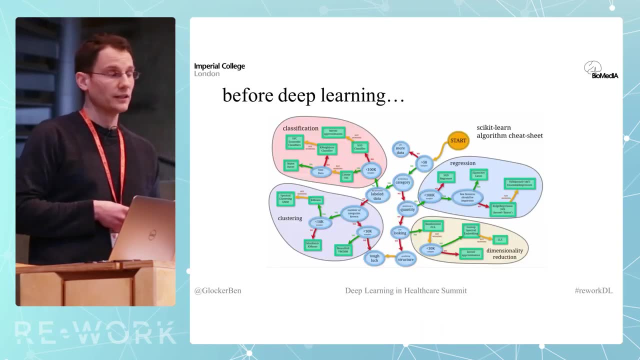 ago. there wasn't really much, And I guess this is the third deep learning summit in healthcare, So you can see that they were right at the beginning of the trend when they started these summits Before deep learning. actually what we were 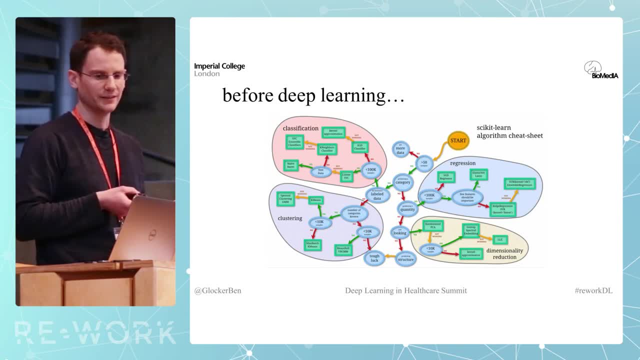 mostly using are more classical machine learning techniques, So I stole here the scikit-learn algorithm cheat sheet. Scikit-learn is a Python library, a very successful, widely used, open source machine learning library. It has lots of classical machine learning techniques. 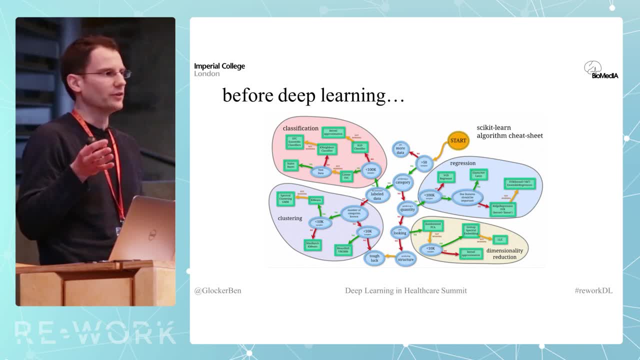 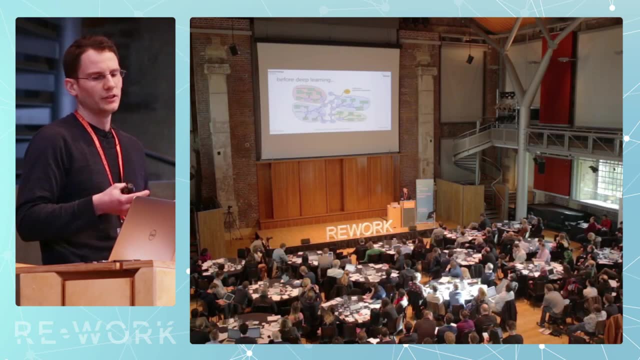 very nicely developed And basically they gave you this guide. So whenever you had a data science problem, you could follow this guide. You could find out which technique to use, Whether it's a classification, a regression, a dimensionality reduction technique, And 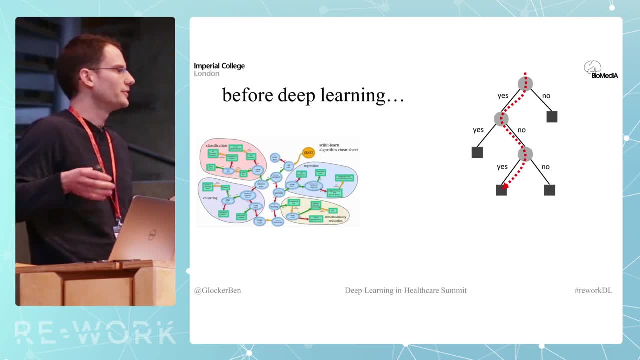 it seems, if you look at the literature now, you can do all of this basically with deep learning. So then, in particular in medical image analysis, a particular technique that we were using quite a lot and very successfully before, deep learning was based on decision. 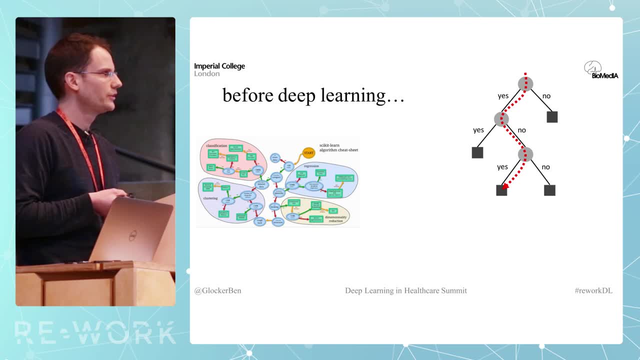 trees. So most clinicians are used to use decision trees And we found ways of using randomized decision trees which were very successful. So that's why we applied to machine learning, added to medical image analysis problems, but also computer vision problems. And the reason why they are nice to use is because 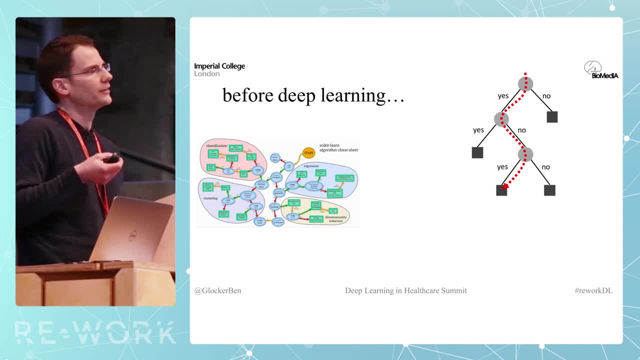 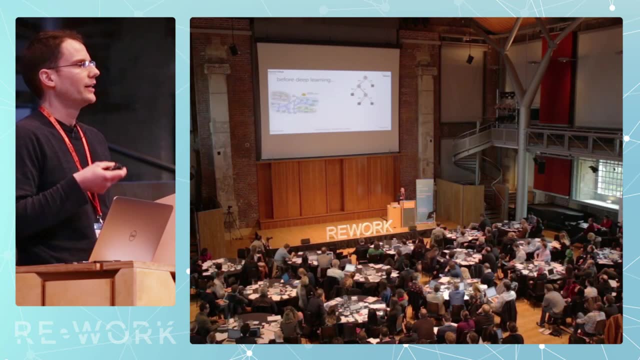 they are quite interpretable. So you have these decisions to make that tell you whether a feature is useful or not, And it can separate your data And then in the leaf notes you can make decisions And at test time you just follow a path in the decision tree And 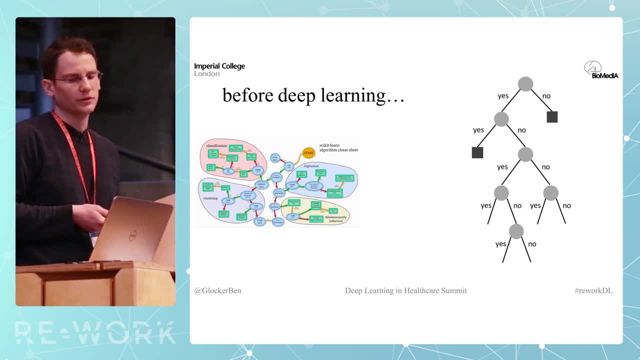 it was very useful. And scaling this up was also quite possible by trying to start building deeper and deeper trees. So you were using lots of features from your data And that, in particular in medical imaging we saw was quite useful. So there was a time before. 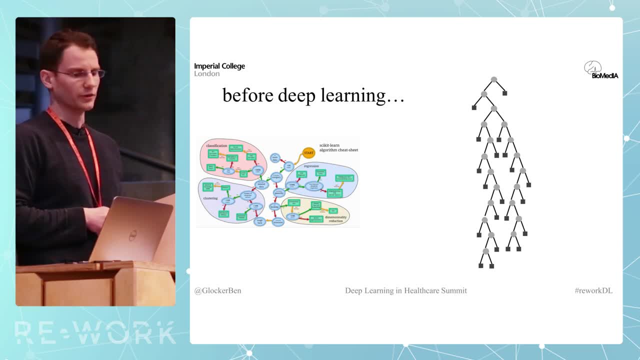 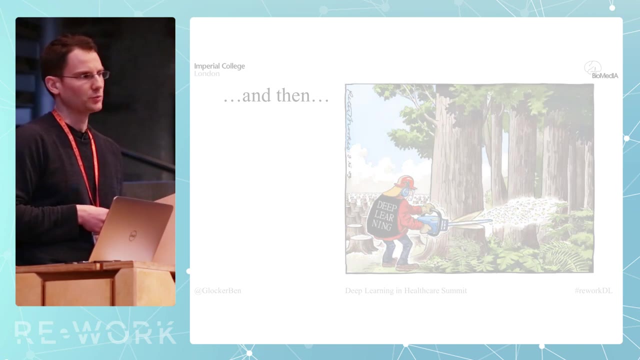 deep learning, where everyone started to use random forests for all kinds of things Because we saw, when we put together lots of decision trees we get very strong classifiers. But then came deep learning And really it has changed the field a lot. So these days people 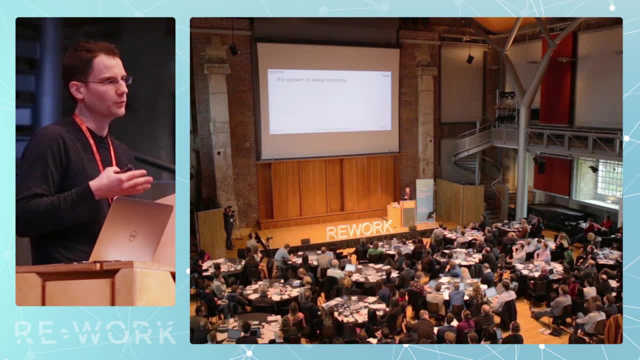 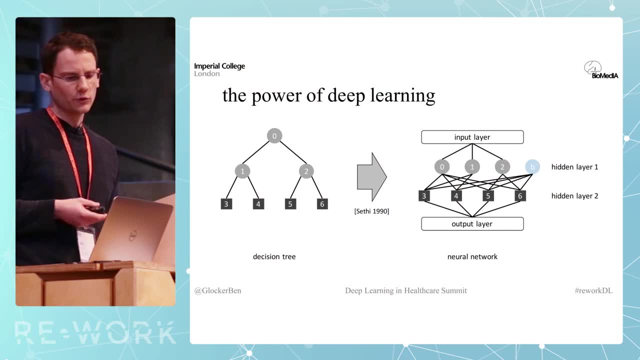 wouldn't consider random forest. They might consider random forest as their first choice. They might just go with a standard convolutional neural network as a baseline to get an idea how difficult the problem is And the reason is why, or where the power of deep learning is really, if you compare decision. 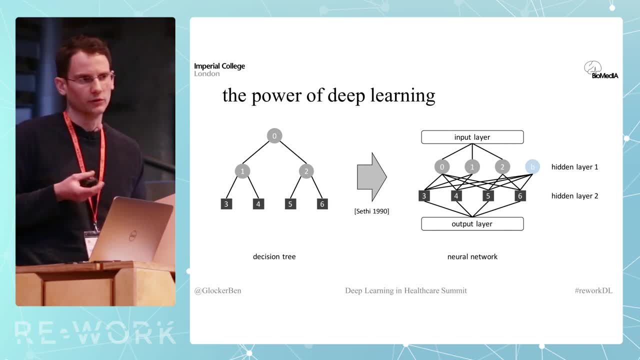 trees, for instance to neural networks, then we already know for quite some time that you can represent a decision tree with a neural network which simply has two hidden layers, So all the decision nodes of a tree on the first hidden layer and all your leaf notes. 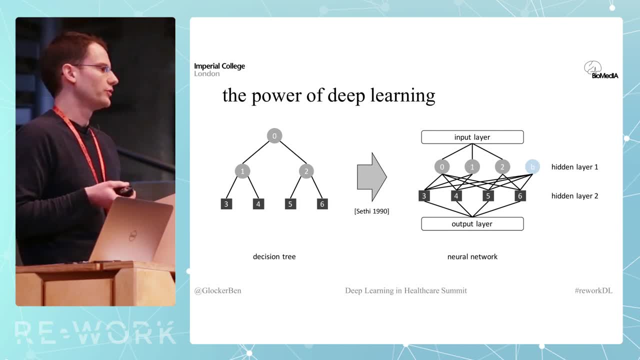 on the second hidden layer And that's how you can perfectly represent a decision tree with a two-layer neural network. Now, if you build deeper trees, where you get the more discriminative predictive power from indecision trees, the interesting thing is to note is 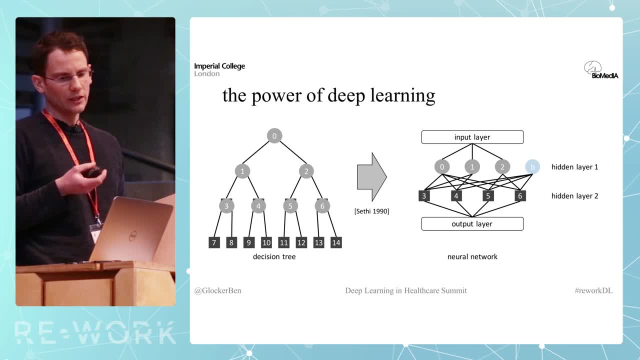 that you don't get deeper networks, You simply get wider networks. So a deeper tree mapped again to a neural network gives you a wider network but not a deeper one, And the deep learning technique is the only way to get the power, I guess, in deep learning techniques. 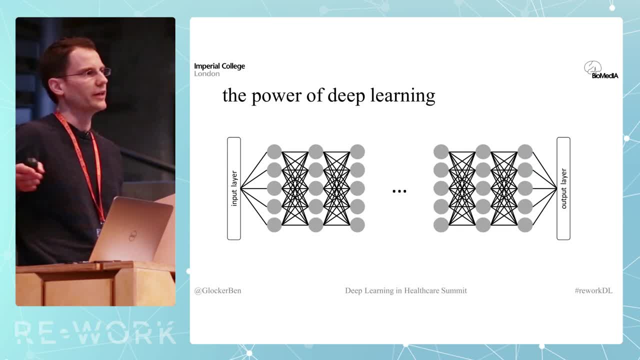 So, if you look at what models are used these days, you have lots of hidden layers stacked on top of each other, And this stacking of hidden layers allows you to learn these very complex data associations between your input data and your output data. And that's where 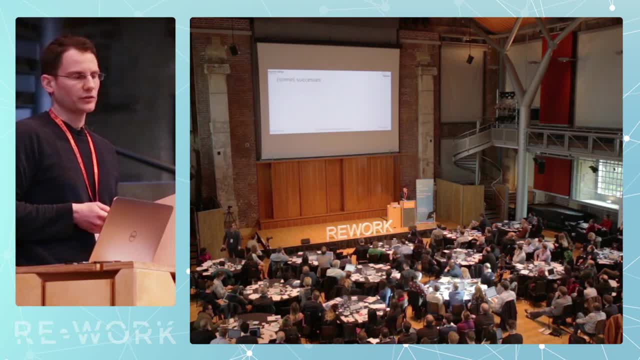 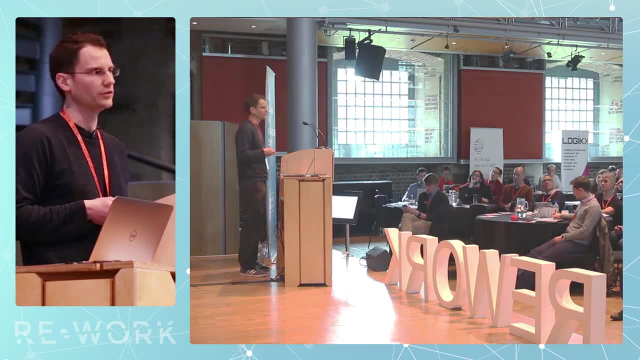 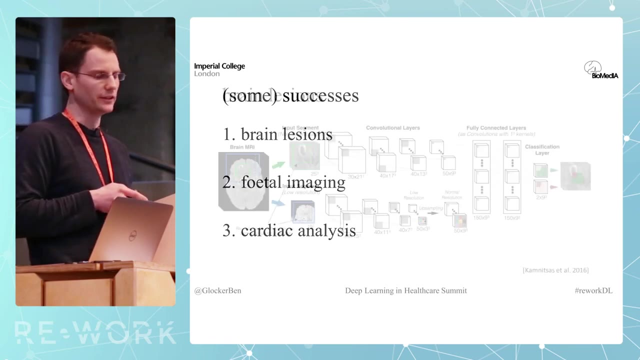 the power is coming from. So just to give you some successes from our own lab where we have applied in the last couple of years deep learning techniques. I want to show you some results from brain lesions, fetal imaging and also cardiac image analysis. So the first one is on brain lesions. So this is work that we have already started. 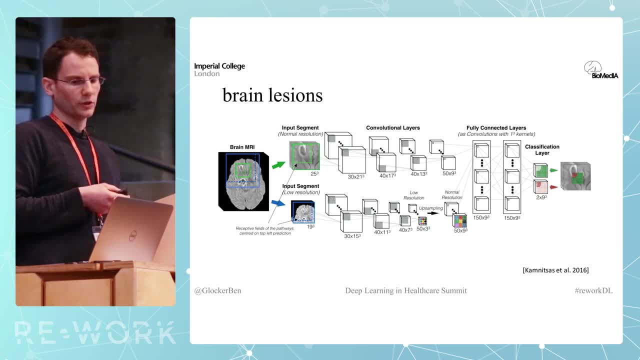 to present last year where we started with this. So one of my PhD students, Kostas- who is here in the audience- if you want to raise your hand, Yes, Because he can answer your detailed questions afterwards- So he came up with this architecture, So we used a relatively 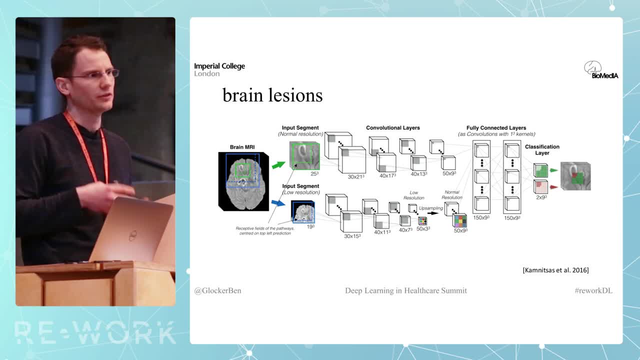 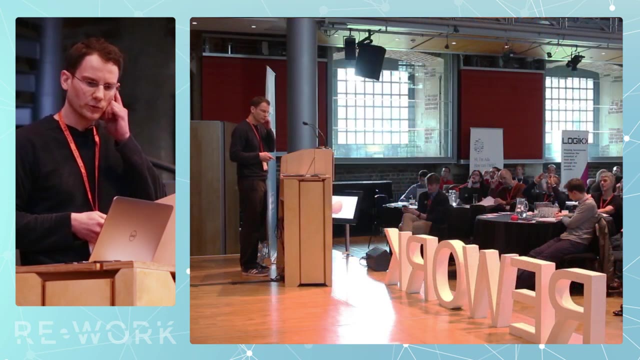 standard convolutional neural network. We made it possible to process large 3D imaging, So this is done on 3D volumetric brain scans- And we used a multiresolution approach because it helped us to incorporate local but also spatial contextual information, And that worked pretty well. So this network allowed us to 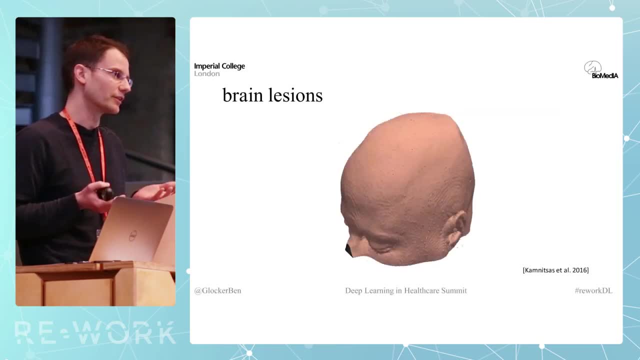 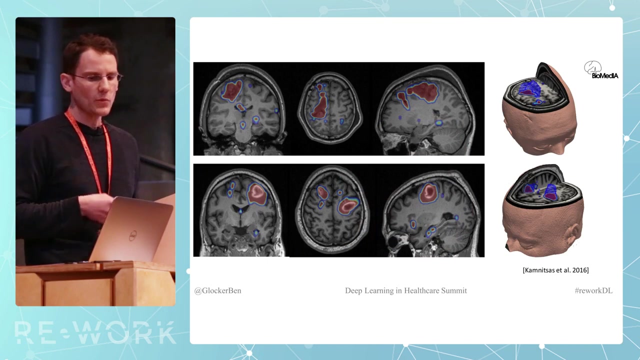 come up with a system that was able to analyze a 3D scan and give us a 3D very accurate map of where the network believes there are lesions. So this was done on brain lesions- people that have accidents And thus maybe have contusions in the brain- But it equally works well for things like 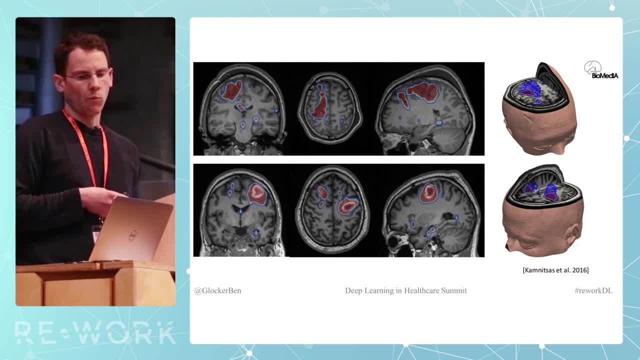 brain tumors or ischemic stroke lesions, And here's just some visual results. Of course, there's a proper evaluation of this in our publications, And using these techniques we found that we can actually apply it to quite other applications, but which are similar in nature. 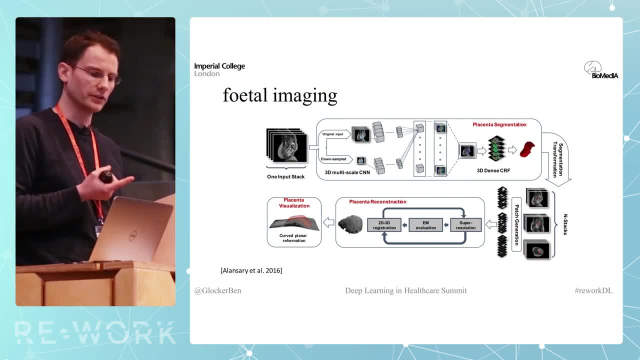 So the next application we did last year. so Amir Al-Azari, another PhD student in our group, used this network for fetal imaging So he came up with an architecture. So this is where the methodology part of a paper goes in, where you describe how your architecture 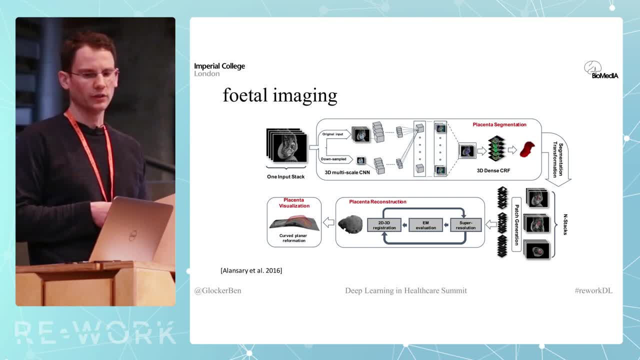 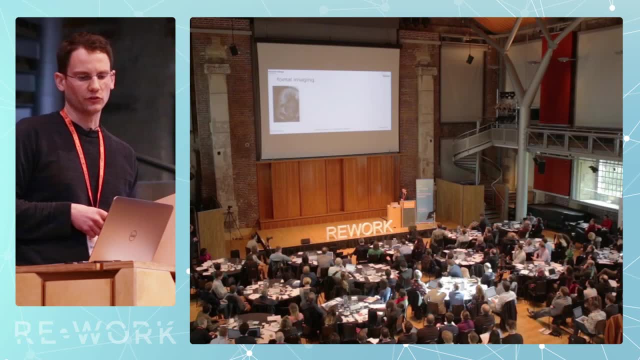 looks like You might do certain adaptations to your previous model. So he came up with a few steps that he needed to process that data in particular, And I'm just showing you some results. So this is again MRI imaging of fetal imaging. So this is a 3D imaging of fetal imaging. 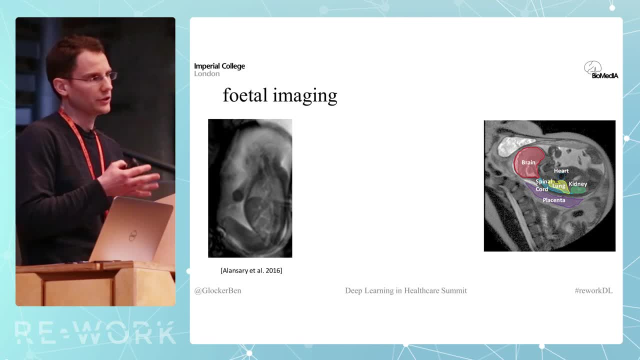 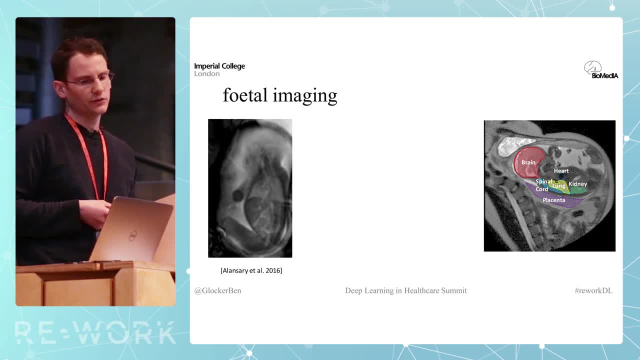 with King's College London, And what we are interested in here really is to analyze these scans and to be able to extract, for instance, the organs of the fetus, because this would allow us to make use of it, for instance, for diagnostic purposes. We want to see whether 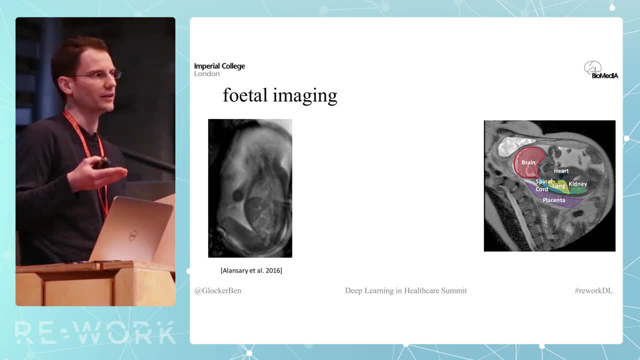 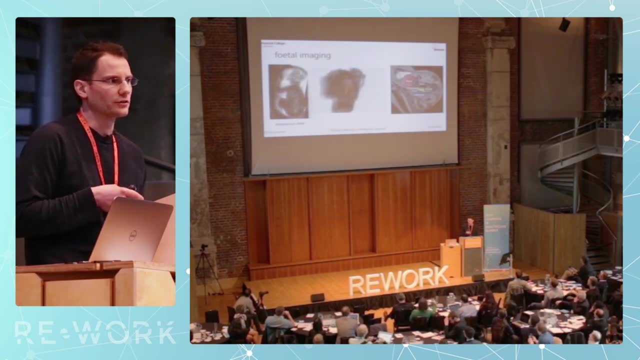 the baby grows at a normal rate. So we want to analyze the brain, the spinal cord, the inner organs. But we also found that with this technique we can do a very challenging task of placenta segmentation. So placentas, the positioning and the shape of the placenta is quite crucial. 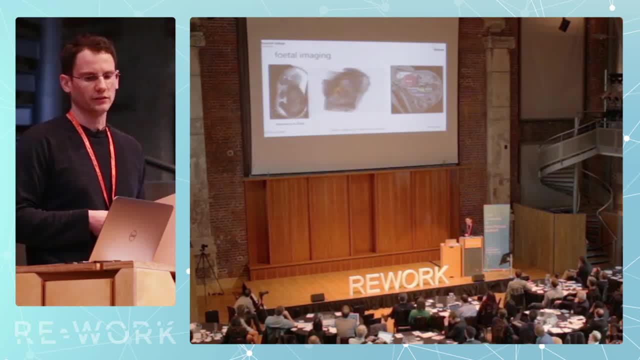 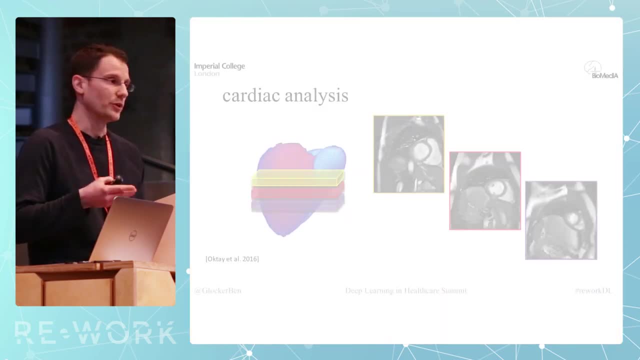 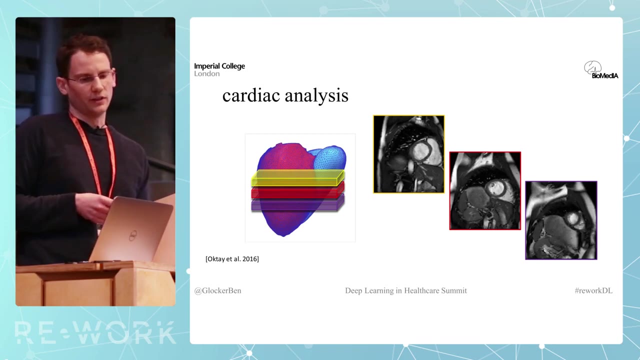 and it allows you to predict whether a pregnancy would follow a normal trajectory. So with this technique we are now able to analyze these 3D scans and actually make use of them in clinical practice. So the next success I would say I want to discuss is cardiac analysis. 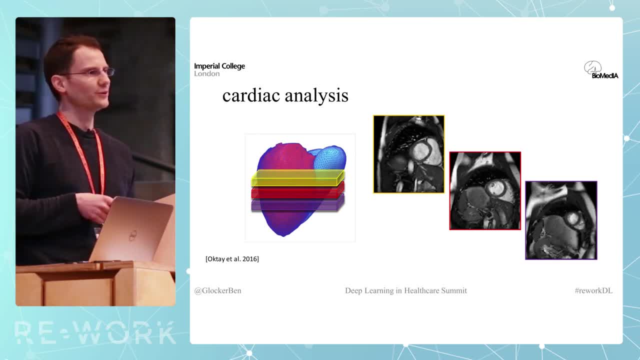 This is work done by Ozan Oktay, who is also here somewhere in the audience, If you can raise your hand as well, So he can answer also some questions. So the problem with cardiac is, if you want to image the heart, it's very difficult because it's always moving. 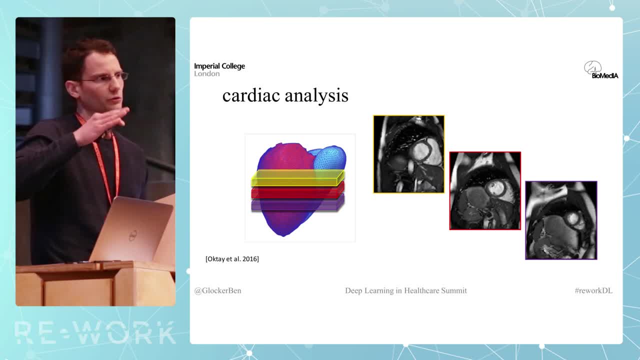 So normally what you do when you again use MRI, for instance, you would do slicewise acquisition, and if you put a slice at a certain position of the heart, you get a slice. You get a nice 2D video, but then at the end what you want is a 3D volumetric video. 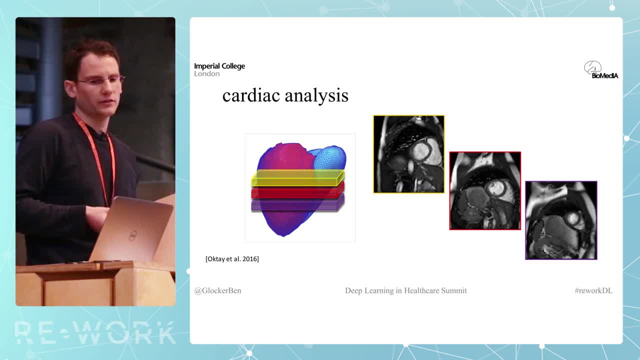 basically a 4D image of the heart. So if you take another slice, you get another video, and you get another slice, you get another video. The problem is you now need to stack them together And because this has to be done relatively quickly, because the heart is moving all the time- 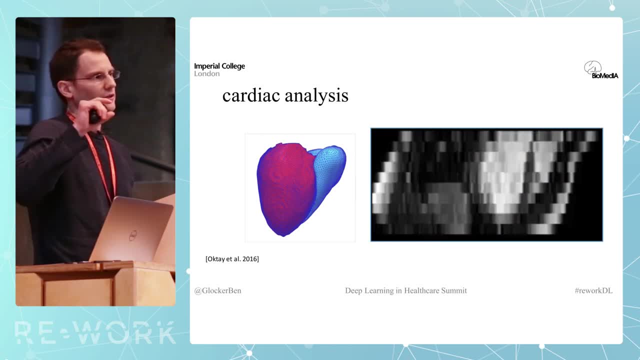 if you just stack them together as they are acquired, you have to use these thick slices, So instead of having a nice 3D volume, you have a stack of 2D slices which are actually quite low resolution if you look at them from the non-scanning direction. 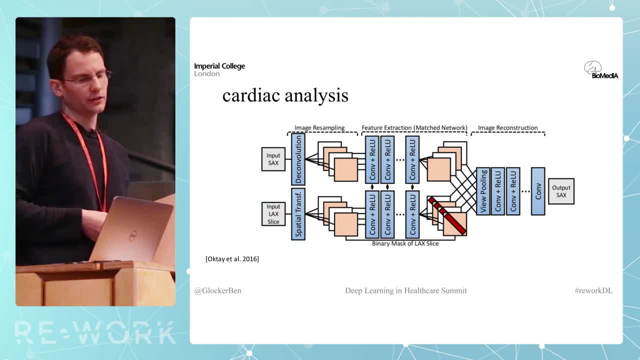 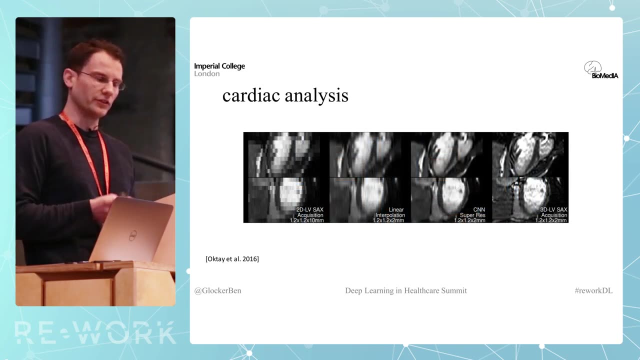 So Ozan was coming up with this network architecture that would allow us to upsample those images. It's a super resolution network. It allows you to basically interpolate towards a higher resolution 3D scan. So here are just some visual results. You see on the left the original data set. 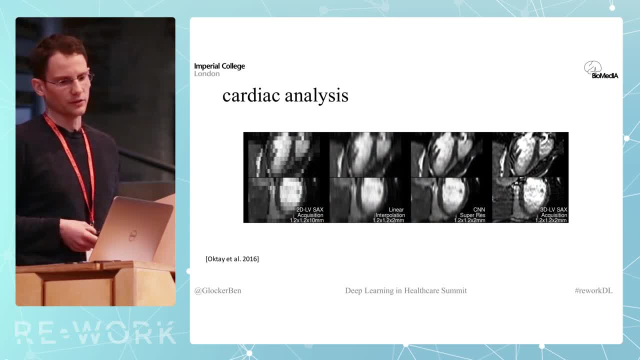 and then you see a standard upsample, Like you're using linear interpolation on the right next to it, And then you see the result coming out from a deep learning neural network And comparing this to a ground truth 3D scan, you actually see that you get quite close. 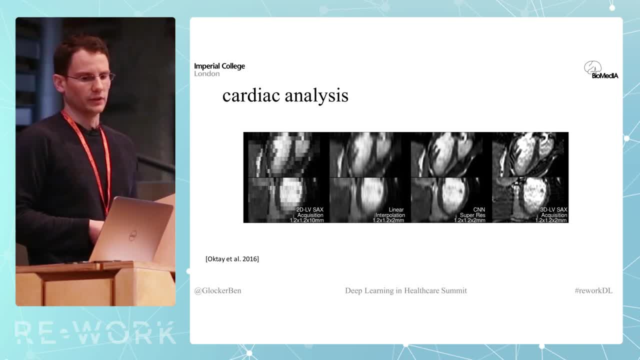 So you even preserve nicely some of the small details. Now you might wonder why, if I can actually acquire a full 3D scan, why would I want to upsample a lower resolution 2D scan? The one on the most right is not something you want. 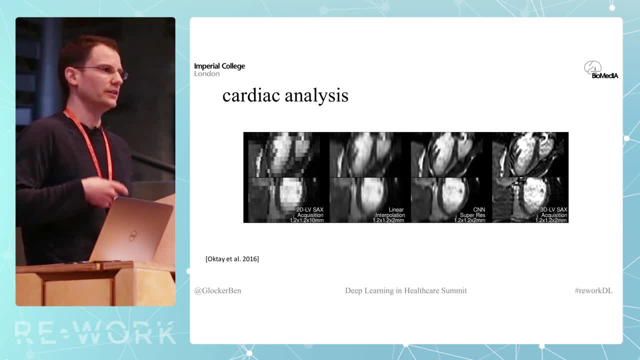 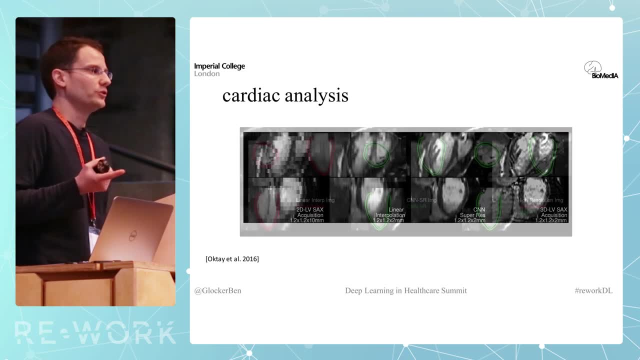 It's something you would do in clinical practice because it takes much, much longer time, It's ECG triggered and it's not something that is used in clinical routine. Now, the images itself: probably you wouldn't use for doing diagnosis because you kind of hallucinate some information. 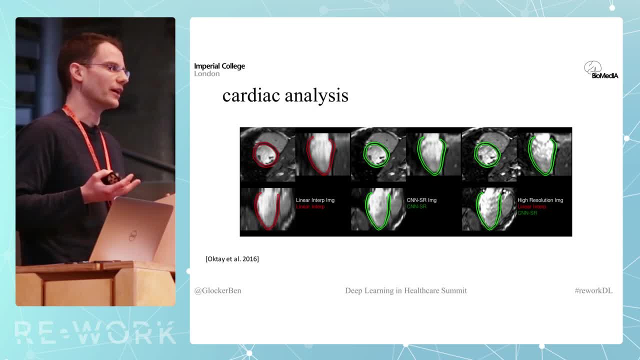 You upsample an image and you might introduce something that wasn't there, So you wouldn't use it for diagnosis. but what you can use it for is further analysis. For instance, we found that you can use it for doing image segmentation, so you can extract the 3D shape. 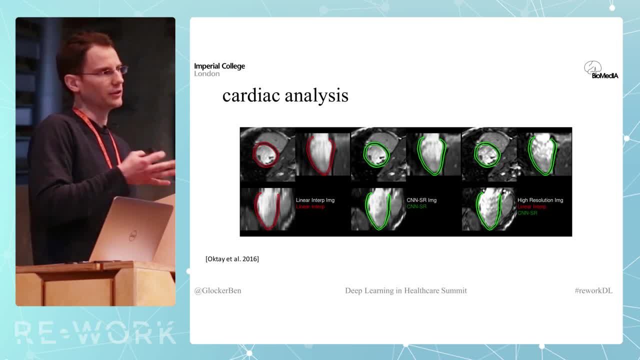 of the cardiac and it's nicer than doing it on the interpolated image and it's very close to the one that you would get on the full 3D high resolution scan. So this you see on the most right. You see, this little discrepancy in red is coming from the linear interpolated image. 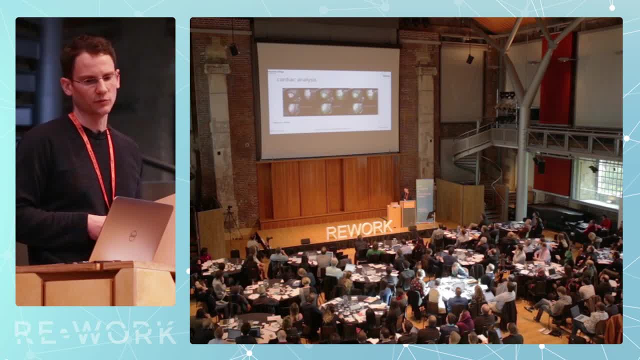 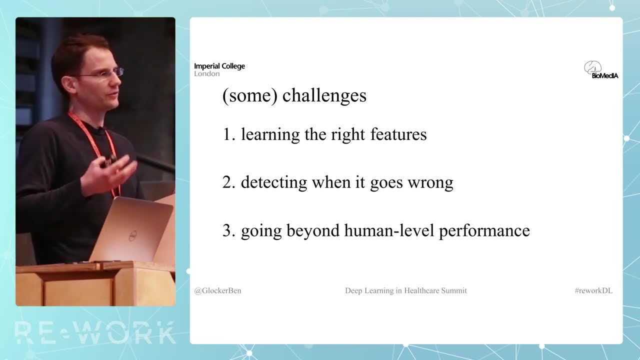 and the green one is from our upsampled 3D image. So this is all nice and we make good success here in terms of we have new applications, applying deep learning on exciting clinical applications. We can write papers about it. But while doing this we also realize that there are quite some challenges. 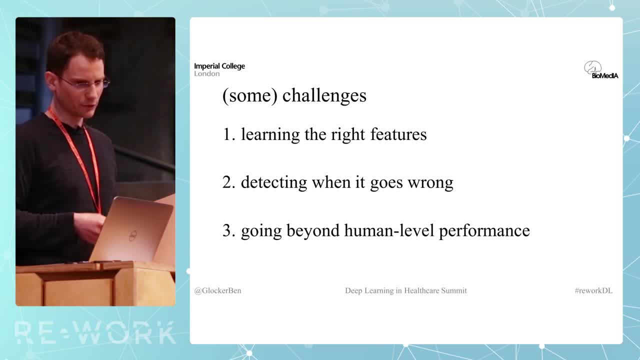 and I guess today there was already a lot of talk about different types of challenges. So I want to discuss three challenges that we saw in particular with respect to medical imaging. So the first one is about learning the right features. The second is detecting when it goes wrong. 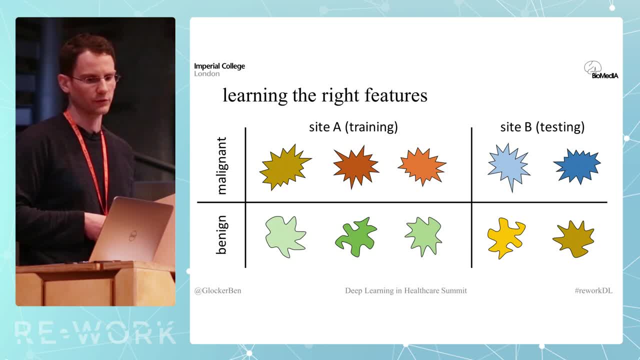 And the third one is: how can we go beyond human level performance? So learning the right features might sound weird in a deep learning context, Because you would hope that your artificial neural network would just do the right thing. So you give it the data. 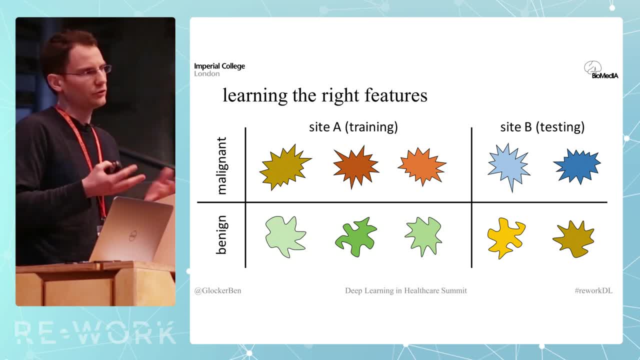 You don't have to worry about hand crafting, designing features. You just let it discover the right features from the data. The problem is with a simple example. I want to show you that that might not always work, So very often, in particular medical imaging, you might get a training data set from a site, one hospital. 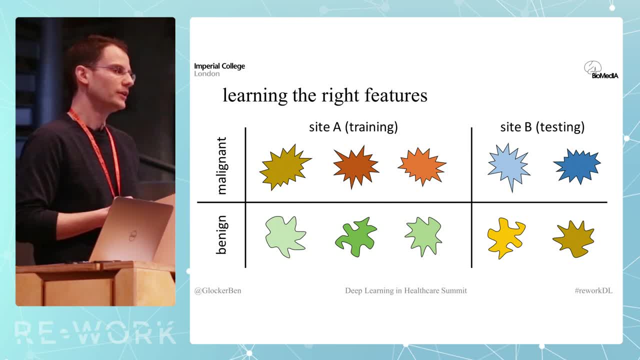 And that might look like this. So you have examples, Maybe even labels. What is the malignant cell, What is a benign cell or structure? And you want to learn features, how to discriminate them. If you give that training data set to a neural network. 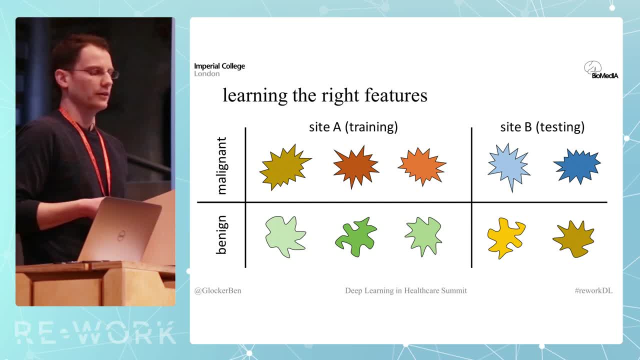 what it will learn is that malignant objects have this orangeness in their appearance And benign things are probably green. However, usually what's happening then when you get new data from another site? you might have data like this, Where you suddenly see that your learned network or your trained network is completely failing on your test data. 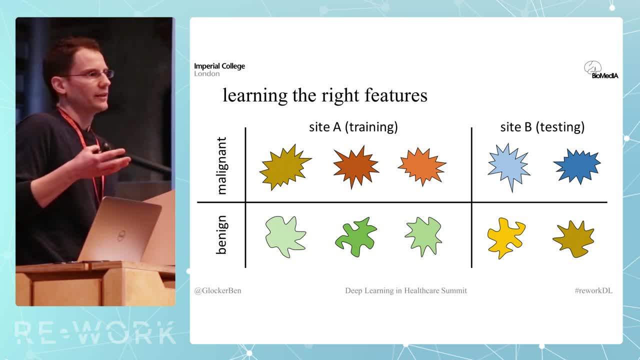 Simply because it learned the wrong features, And there's nothing that would stop the neural network to go for color because of the most obvious discriminative feature in the first place in your training data. Now you might say that's a problem with your training data. 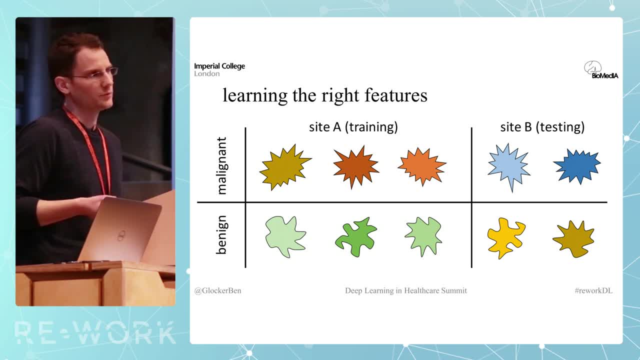 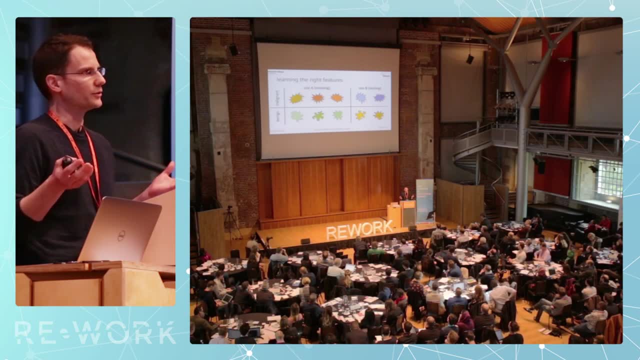 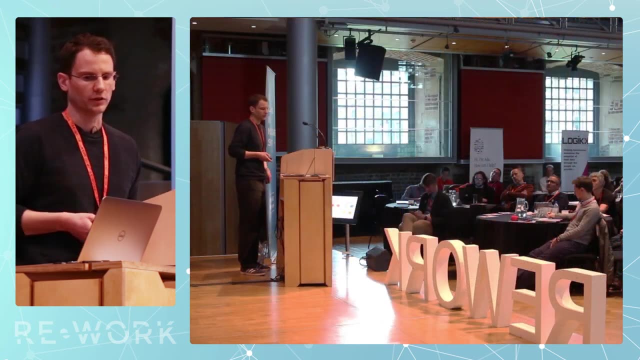 And yes, that's right, That is a problem with the training data, But in medical imaging it is simply not possible to always have a data set that is representative of every possible source of data. There might be a new scanner coming up that didn't exist when you have built your product. 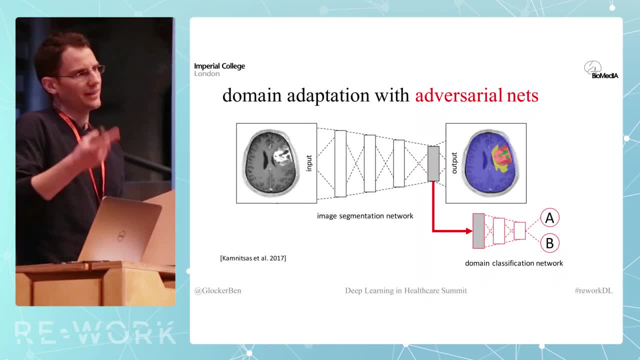 So Kostas again worked on extending his convolutional neural networks by using something that we just discussed a little bit, which is adversarial nets. So we used this to do what we call unsupervised domain adaptation, or what is called unsupervised domain adaptation. 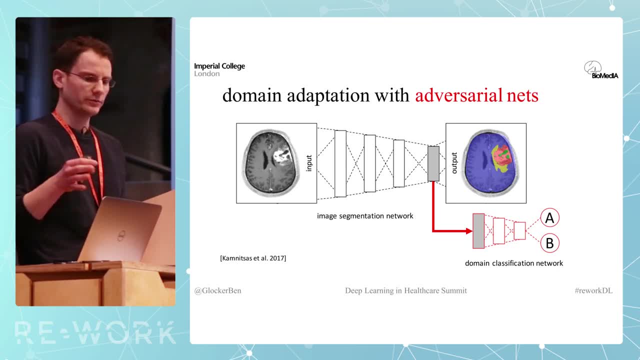 And the idea here really is that if you learn your standard neural network- so let's say you want to do brain tumor segmentation- you learn a network, an image segmentation network, a convolutional neural network that does this. Now, at the same time, what you try to do is you have another network. 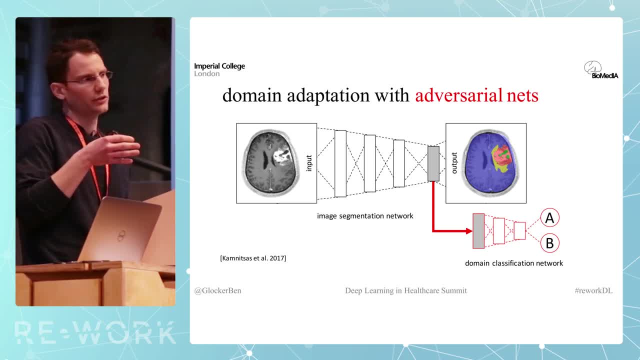 that looks at the learned representations, and what you try to do is you try to figure out where the data is coming from. Now, if you train such a network on labeled data that is coming from your state A and you have another data set that doesn't have to be labeled, 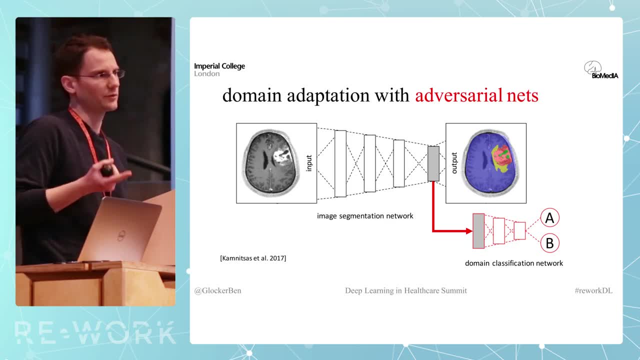 which comes from site B, that first network, the image segmentation network, will try to learn features which are invariant to where the data is coming from, And this allows you to mitigate exactly that problem. It wouldn't learn, for the previous example, that color is the discriminative feature. 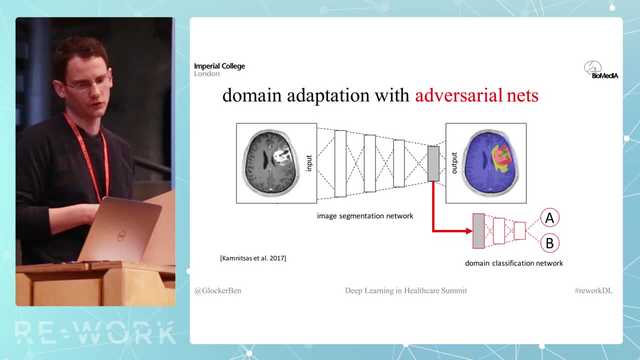 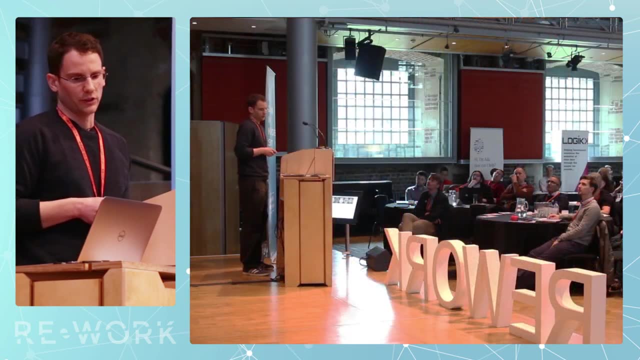 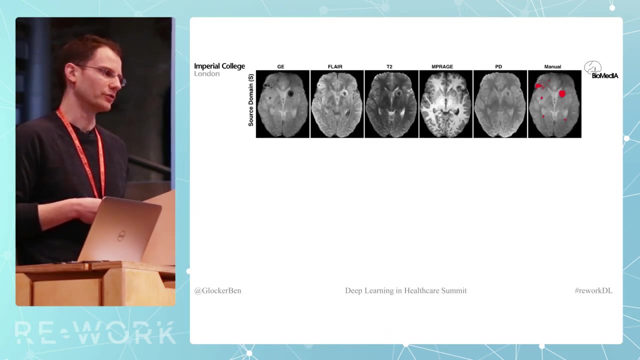 It would learn that it's actually the shape that would discriminate the two structures, because that's what makes them invariant, and invariant to where the data is coming from. So this worked really well. so we tested this again on brain lesions, where we had MRI brain data coming from different sites. 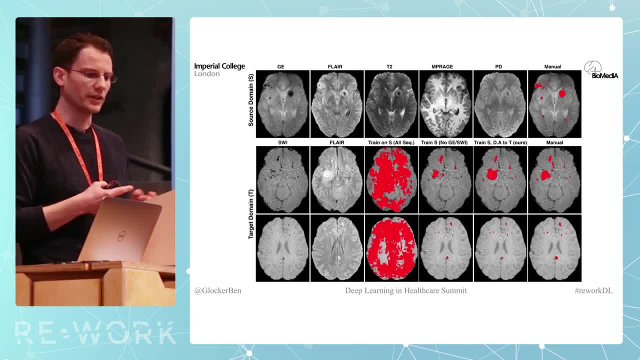 so basically two different MRI scanners And in one of them they acquire a certain set of MRI sequences and in the other one they almost acquire the same, but there was a slight difference because they changed to a new sequence in the MRI acquisition which actually made our previous network that was trained. 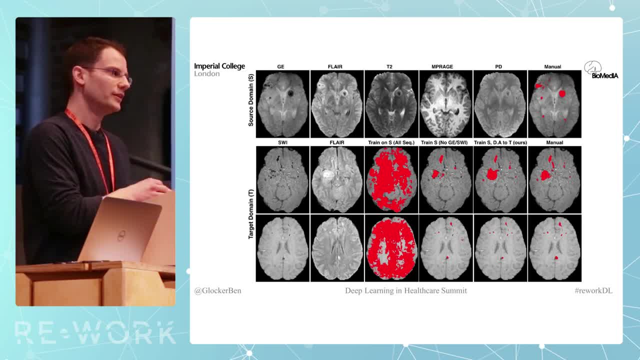 on data from the one scanner, completely fail on the second scanner. However, after using the domain adaptation, using the adversarial nets, our network went up to the performance that it got on the first site, even on the other data from the new scanner. 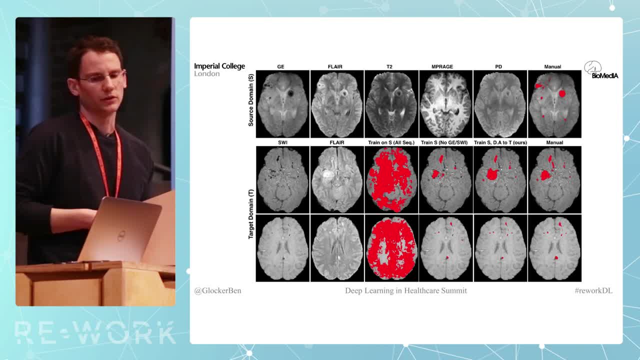 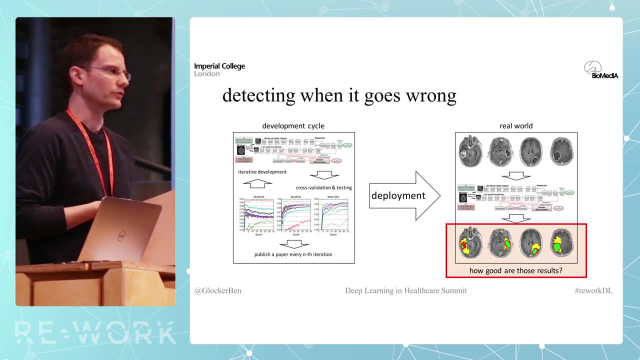 without using any annotations. Just training the network to discriminate or to not discriminate where the data is coming from helped us to get back to the performance and learn the right features. So the second challenge is about detecting when it goes wrong. So very often when you build these neural networks, 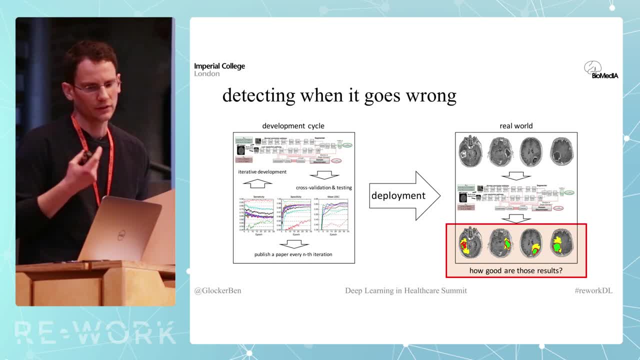 the problem is: you have this development cycle. You build a neural network, you do validation and testing, you look at your learning curves, you do modifications on your network and you live in this cycle. So, at least in academia, we often live in this cycle. 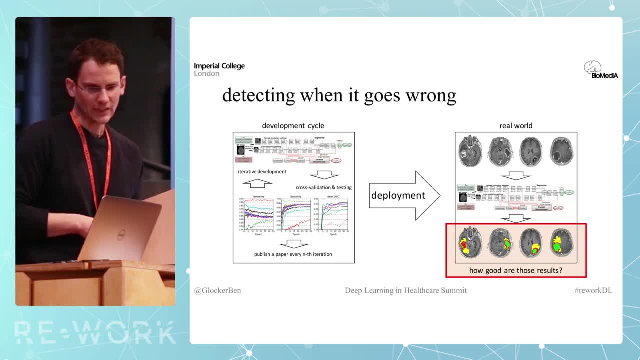 and then every end iteration we try to publish a paper. Now the problem is, at some point you want to use those systems in clinical practice. So if you go to the deployment and you use now a trained neural network on data that is acquired in the hospital, 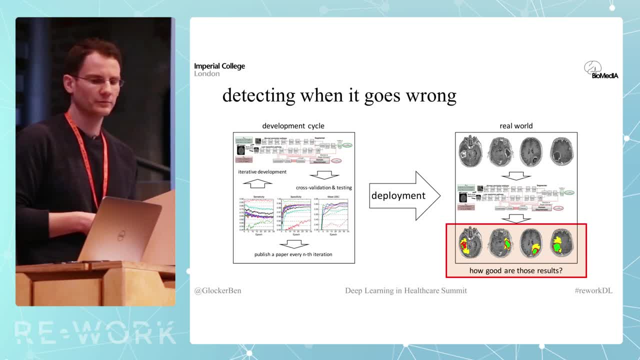 what you might find is that it doesn't work so well. The problem is: how do you know? How do you know that it doesn't work well? You could look at the images and you could try to do some sort of manual quality control. 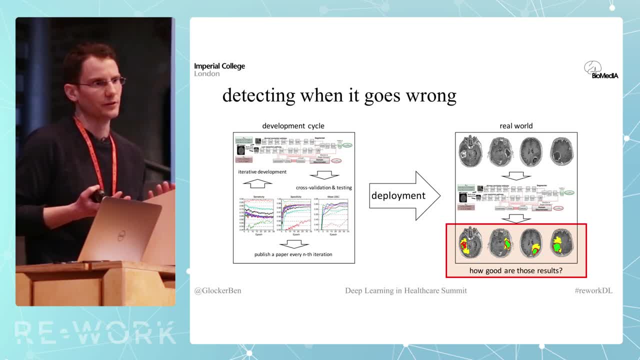 you could annotate data, but that's not feasible at scale. You can't always look at. if you have a large scale data analysis, you can't look at every single case and check whether your network worked well or not. So what we are trying to do here is basically: 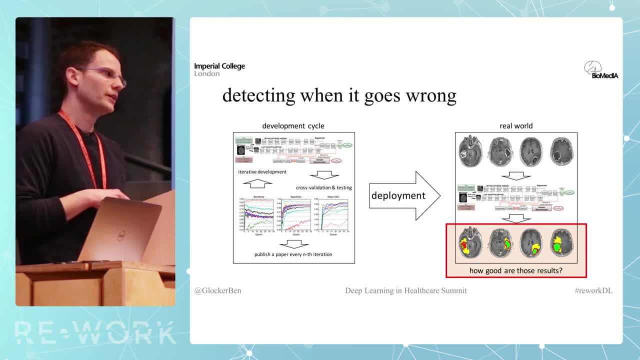 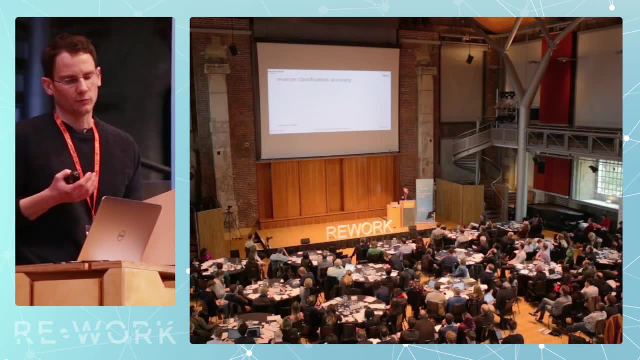 we try to figure out, to automatically recognize when something goes wrong, But not on average but on a per subject basis. So we came up with this framework- reverse classification accuracy- which is of course, based on previous work on reverse testing and reverse validation. 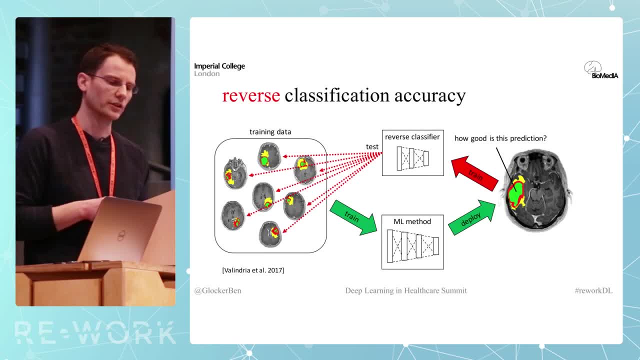 But really the idea here is to use this within a medical imaging setup where we say there is normally some training data, some reference data for which we know what the true labels are, at least the ones that we believe are the best possible we can get. 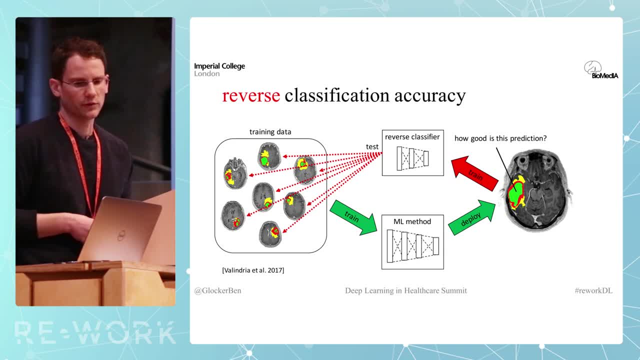 Those are usually used to train a network. so you learn a system, you learn a machine learning method, a convolutional neural network, something that you can then deploy in practice. Now, on your new data, you get a prediction, and the question is: how good is this prediction? 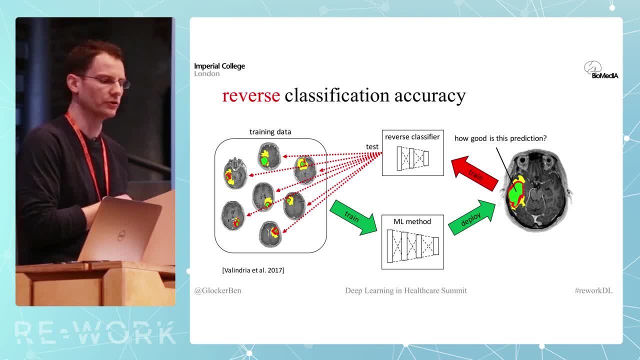 Every time you want to know did it fail or did it do a reasonable job. You can use the prediction and train what we call a reverse classifier. So that is a classifier that is completely overfitted to that one example, But you can use it to make predictions again. 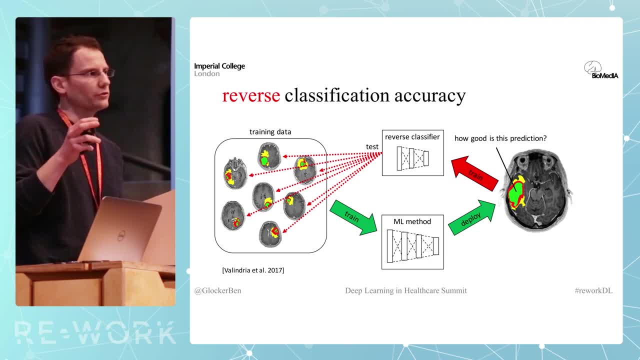 because it was trained on so-called pseudo ground truth. so something on a prediction. So now, if you go back to your training data, you can actually check how well does the reverse classifier work on your training data. And of course, it might not work well at all. 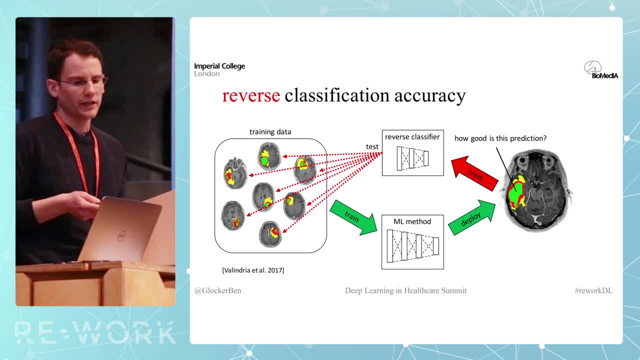 and, in particular, it might not work on all of them, but it might actually work on some of them. And it might work on the ones that are very close to your testing data. And now, on this one, you can actually, of course, quantify, you can get a number, a quality score. 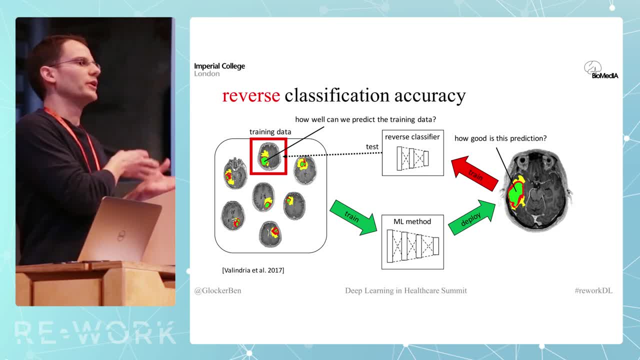 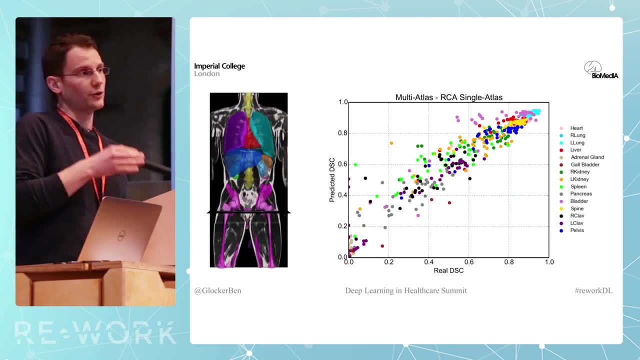 a metric that tells you how well could you segment the training data by using the prediction in your test data, And we show that this is actually well correlated with the true performance that you would get on your test data. So we tested this on multi-organ segmentation. 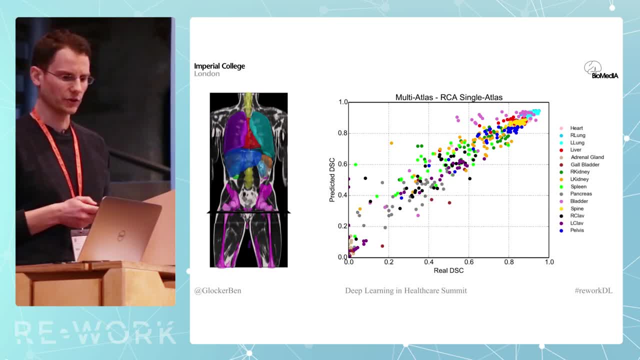 in whole body MRI, but in the meantime also on cardiac imaging, But just to show you a plot. so this is on the x-axis, the real DICE score. so it's one segmentation quality metric that measures overlap between a predicted segmentation and a ground truth, manual segmentation. 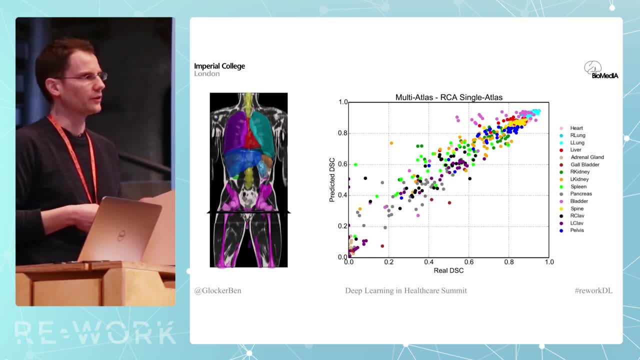 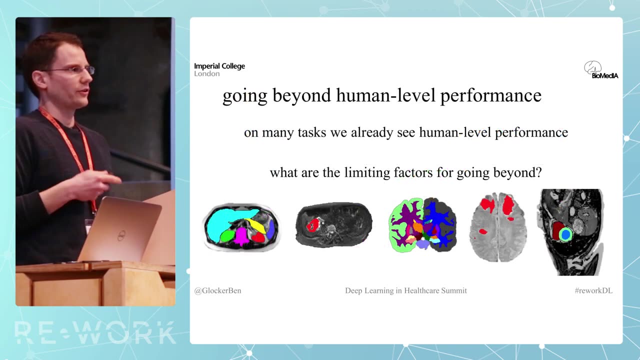 And you see that the predicted score that we get automatically correlates very well with the real score. So you could use this, for instance, to automatically detect, by setting a threshold, for instance on the predicted score, if a system has failed. So now the last challenge I want to discuss. 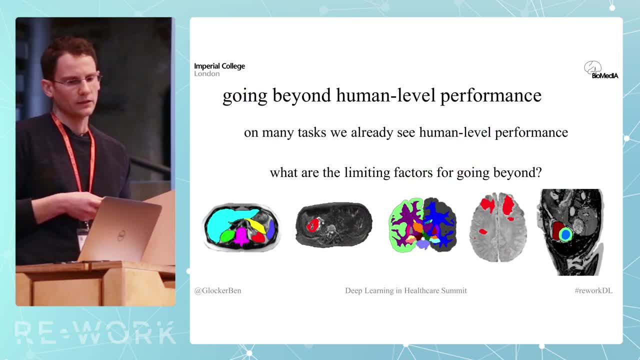 is: how can we go beyond human level performance? Now we already see, although there's a lot of talk about reaching human level performance for many tasks, but the question is: how can we go beyond and what are the limiting factors, in particular in medical imaging? 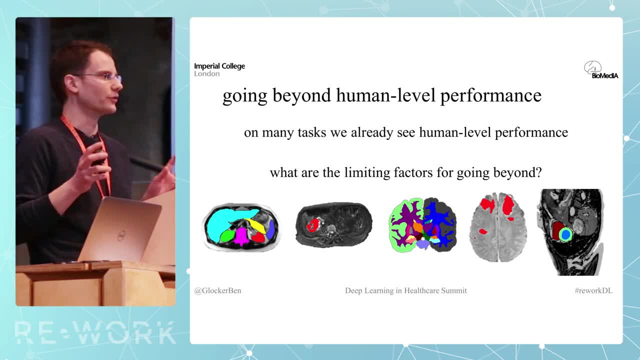 Now, obviously it's somewhere in the data that is generated where we say we have ground truth. we never have ground truth. we have something that an expert provided us. So we try to find the best expert we can, but still, of course, there will be a lot of variation. 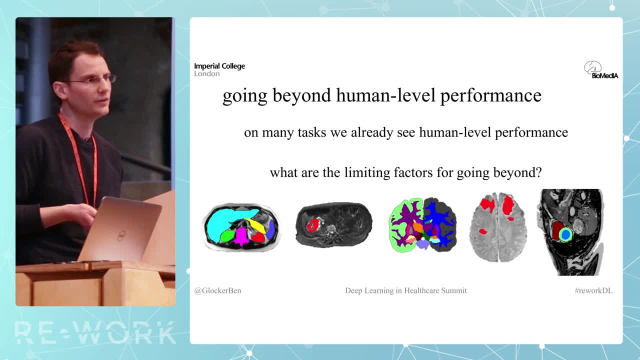 in the quality of annotations. So they have to sit down and have this very tedious and time consuming job of very detailed annotations in medical imaging. And, of course, if we train methods that aim to replicate this, it's very difficult to go beyond. So you can maybe reach the performance. 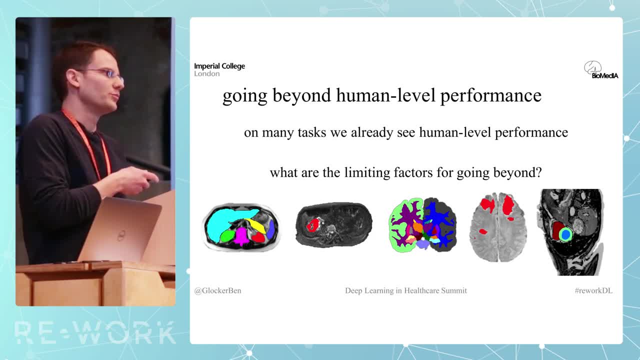 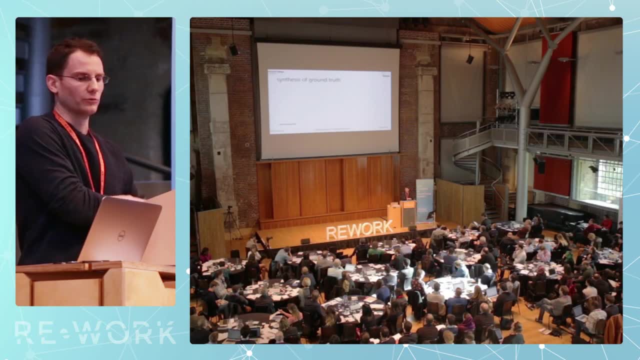 of the best expert, but ideally, at some point we want to use this to be better than humans. So one idea of this- or I think one direction promising direction would be- is to really think about synthesizing ground truth. We don't want to rely on experts and their time. 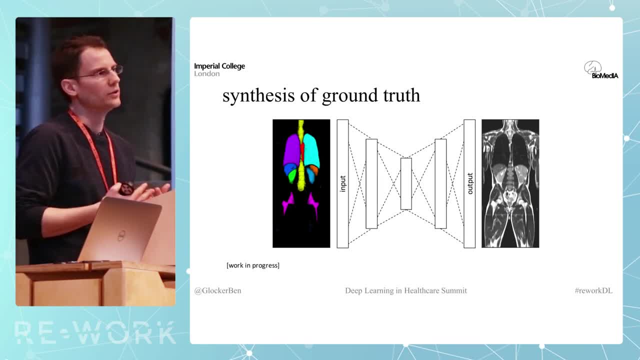 and doing the annotations. we want to generate data for which we know the ground truth, And this could be done by synthesis. We have, I think, heard about GANs, which are one way of synthesizing data, and we have seen maybe all science. 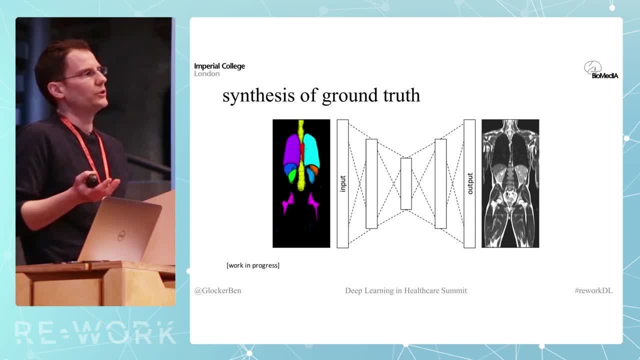 from recent works on that. So the idea would be really what if we could draw a manual segmentation label map and have a network that would produce us the corresponding image, Because then we really have the matching input and output data And it could be considered ground truth.